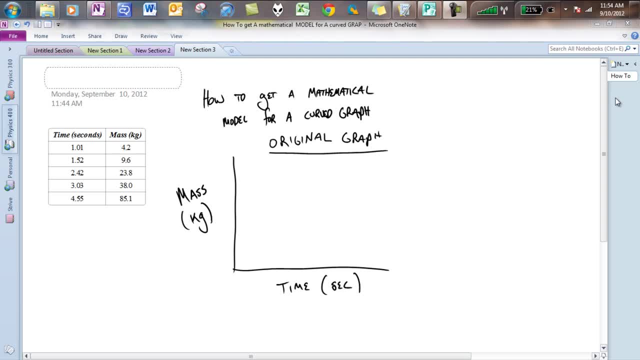 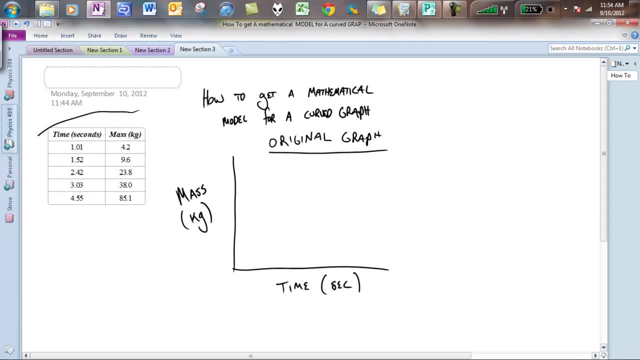 You might want to just take a couple of quick notes just to remember where these buttons are. I'm actually going to do example number three of the worksheet. You can see the data table which I have listed right here. All that you do is you'd open up Logger Pro and you would type those values in. 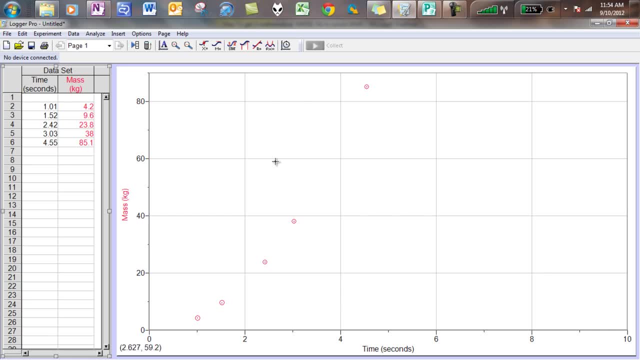 Again, you can see those values typed in. Whenever you do this, the first thing you should do is right-click and go Auto Scale. This is what my graph looks like. If I was doing this for a test, of course, I would draw in those points. 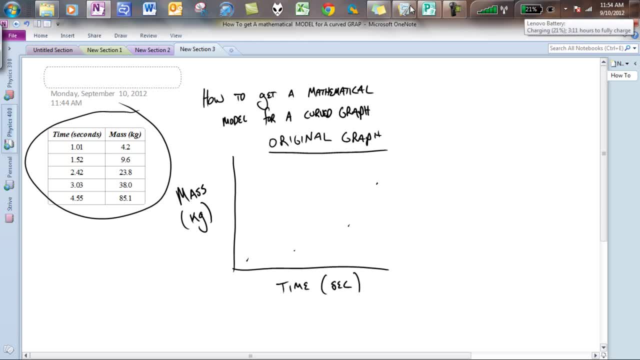 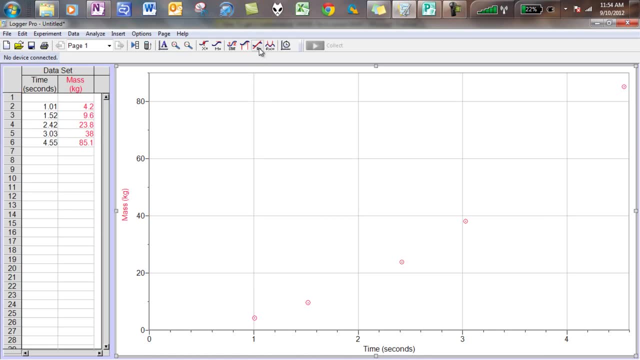 The first thing that I noticed when I drew in those points is: yeah, looking back at the graph, take another look. You'll notice that it is curving upwards. That's a pretty telltale sign. However, before I do anything, I of course want to analyze the correlation and RMSC. 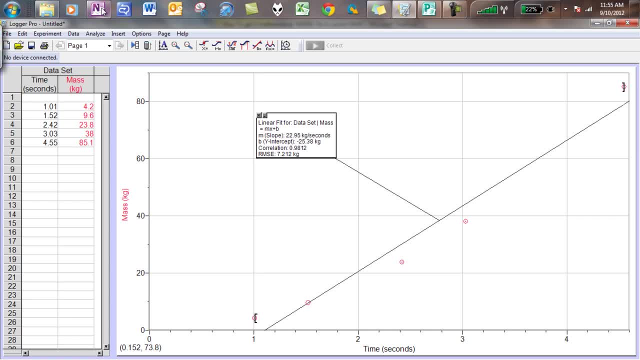 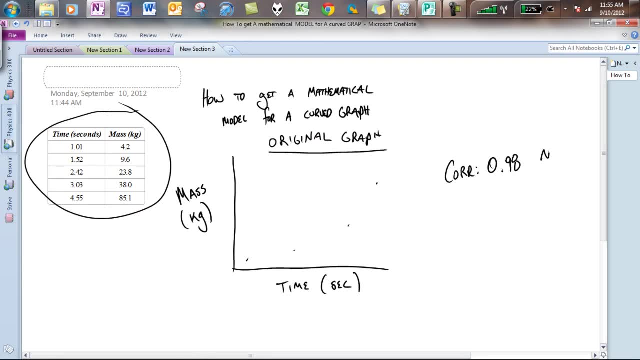 I look at the correlation and I see 0.98.. I'm going to go here and I'm going to say: the correlation, The correlation is 0.98, and that is not good. Remember, we want 0.99 or better, so that does not fall under our standards. 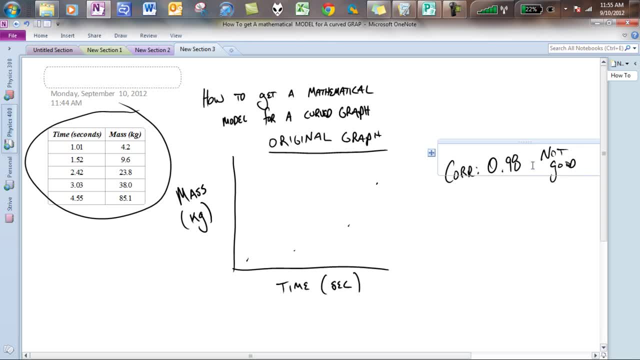 That's one thing against it. Just because it has one thing against it doesn't mean anything bad. It just means that we have one thing that's telling us that maybe this is not a straight line. Second thing that I would look at in this case is the RMSC. 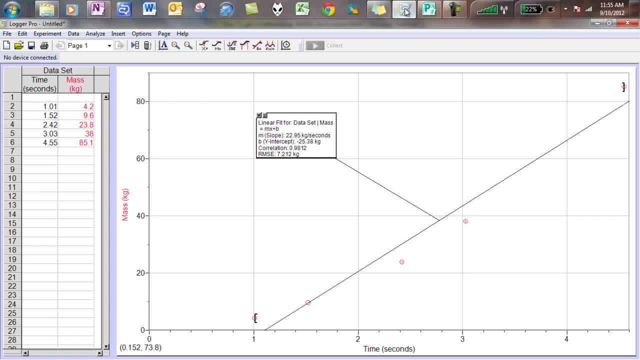 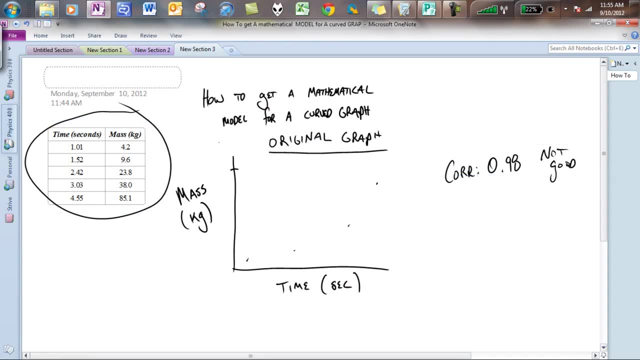 First off, the RMSC is 7.2.. I'm noticing my highest y-value is 80, so let me go back in here. Let me write those things down. I'm going to label this as, again, I believe this was- highest point was 80, and if we take a look, it was about 85.. 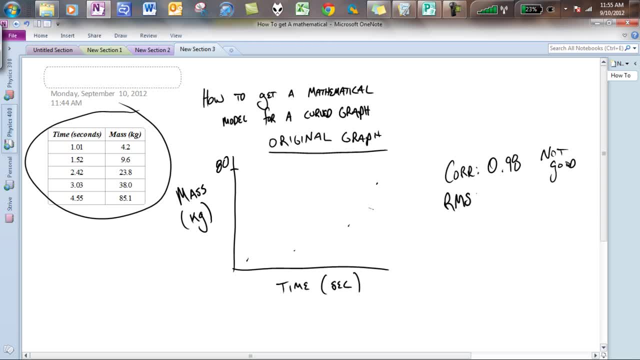 I'm going to call it 80, and our RMSC. let me just double-check and make sure I go back there. RMSC, you can look on there. It's a 7.2, so let me write that down as 7.2. 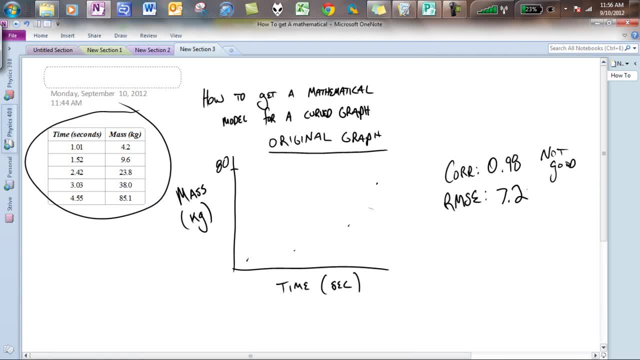 Again, we would want to use our RMSC. We would want to use our RMSC standard and say I will give myself 2.5%. So in this case, if we think about it, 0.8 is going to be 1% of 80.. 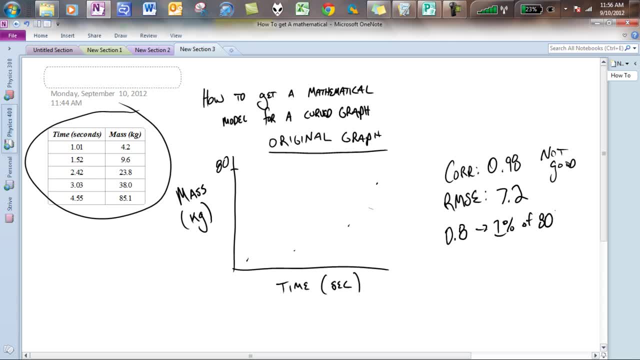 So 2% is going to be 1.6, and if we look at this, this is actually going to be 2.5% of it, 2.5% of 80.. So this is going to be 2.0.. 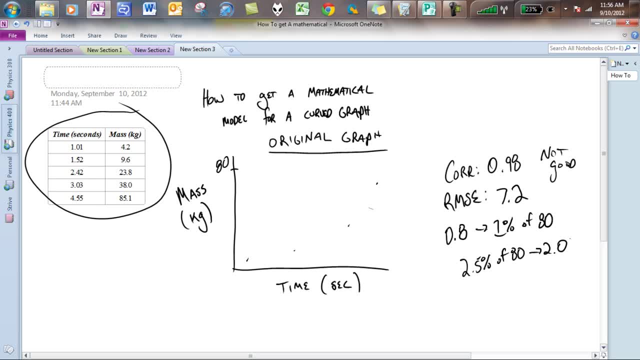 And we say: I'm giving myself 2.0 in terms of error and my RMSC tells us how much error we have and you'll notice it's 7.2. So we are off. We are not within our window, so this is not good. 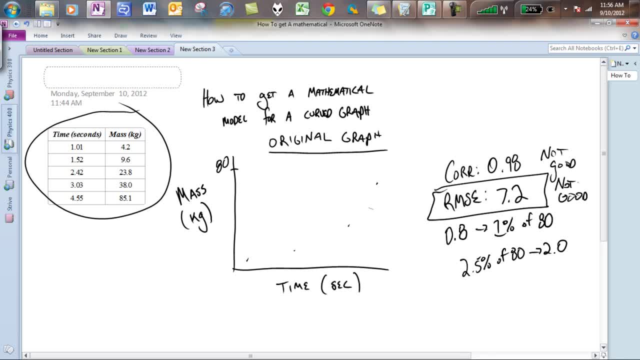 So right away I got two not good things out of here And, of course, the third one. if you actually drew in the best fit line, you notice that it goes under, over, over under. That was a horrible best fit line. 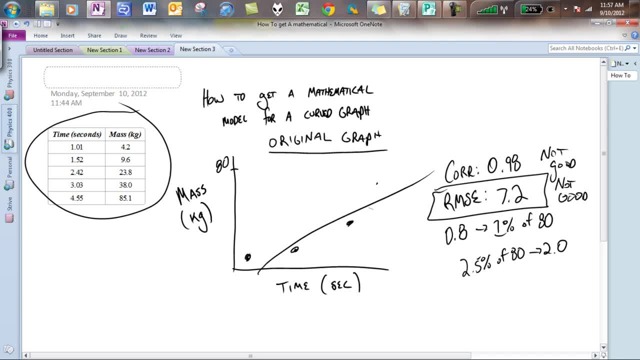 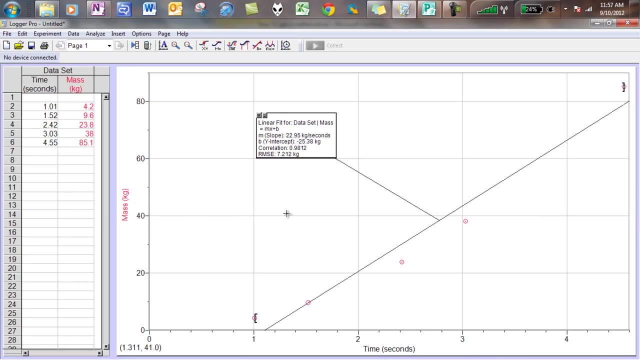 It was more like this: It goes under, Over, Under, Under Over, And you can just see the curve out of it. So right away you'd say: you know what? This is probably not a straight line. So the next thing that we would have to do is go back to the graph and say, well, what type of curve is this? 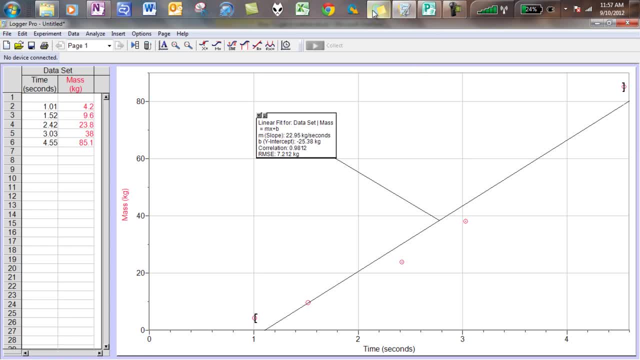 And if you look at your best friend, I think we can all agree that it looks like it is curving upwards, very similar to an x-squared graph, And so in this case we know that it tells us to graph 1.. 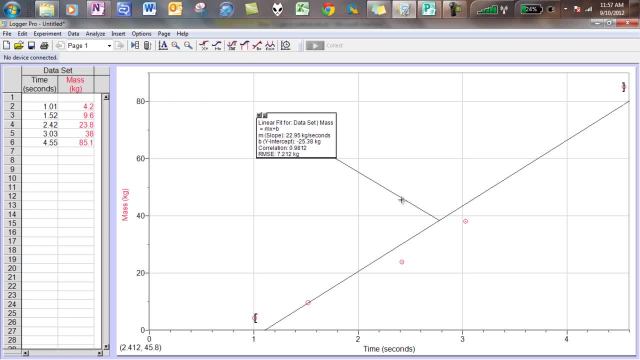 It tells us to graph y versus x squared. So now I want to graph mass versus time squared. So my time axis, which is right down here, I want to change to time squared, Or in this case, you see the time values here. 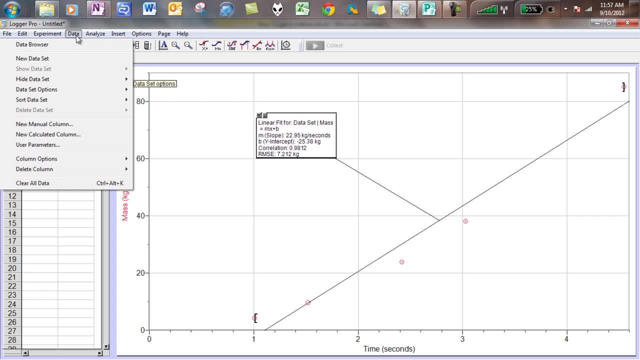 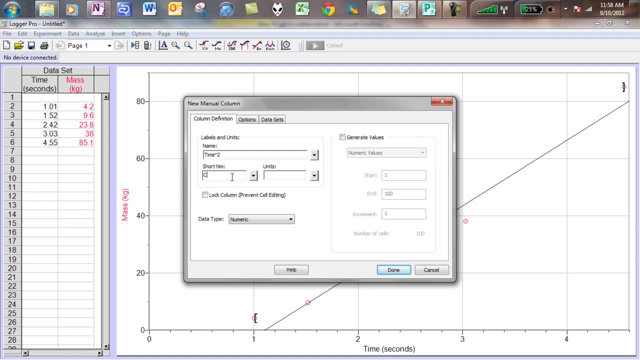 I want to square all those. So in order to do that, I go to data, I go to new manual column. I call this time squared Short name. We're not doing short names And remember, we need to square the units. 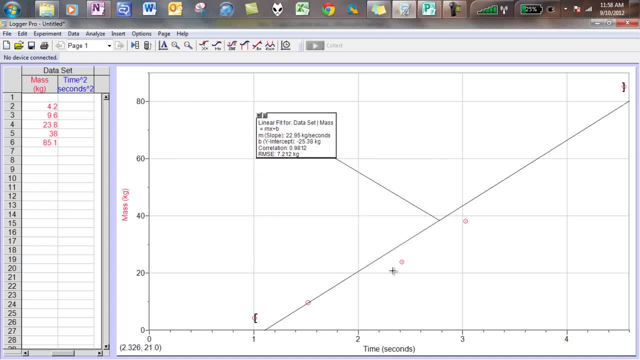 So this is going to be seconds squared. If we plug that in there, you'll see a new column pop up, And all that I want to do right now is to take my time values and square them. So, with a calculator, 1.01 squared is going to be 1.02.. 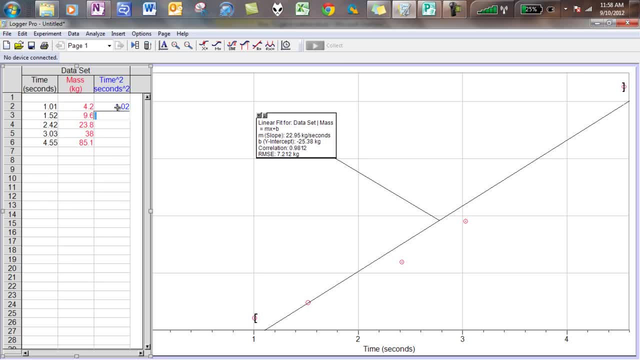 And again, sig figs probably should follow them as you go through. So 1.52, square it, We have 2.31.. And you just go through here real quick And you're squaring all of these values, plugging them in on over here. 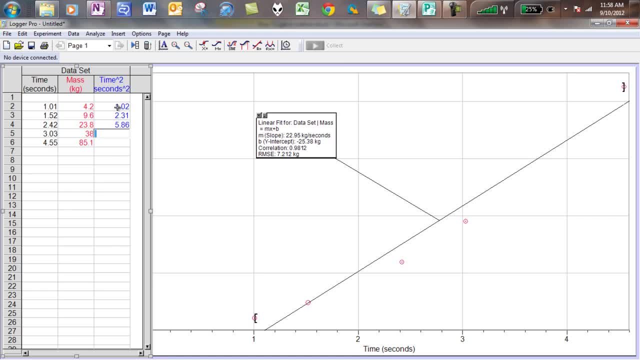 5.86.. 3.03,, square it 9.18. And 4.55, squared of course, is 20.7.. So we look at that And when you plug this in, you realize that nothing's really happened. 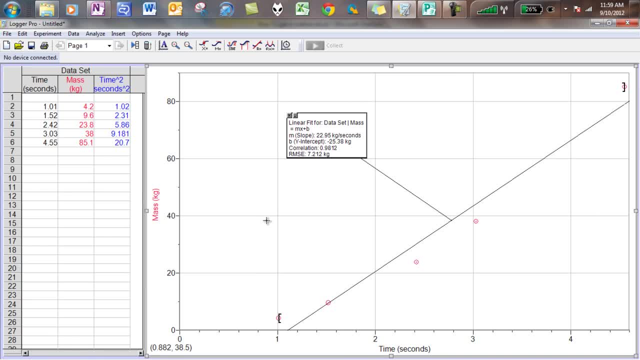 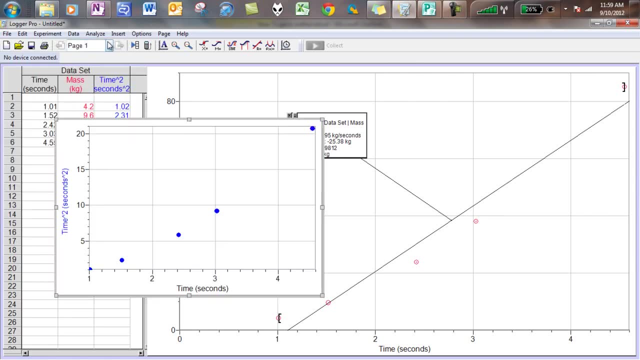 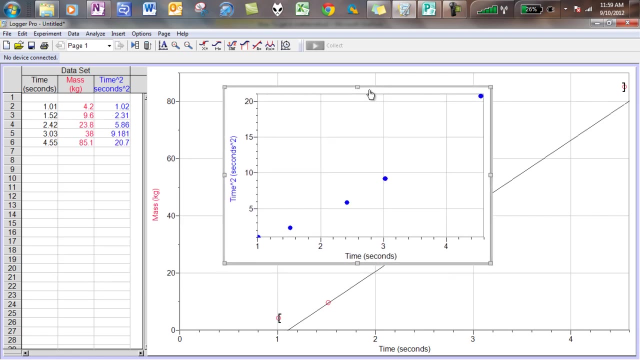 So the next thing we're going to do, the next thing that I'm going to want to do, is actually graph it. So I go to page- I'm sorry, insert. You go to insert a graph And right away you notice that this graph that was inserted is time squared versus time. 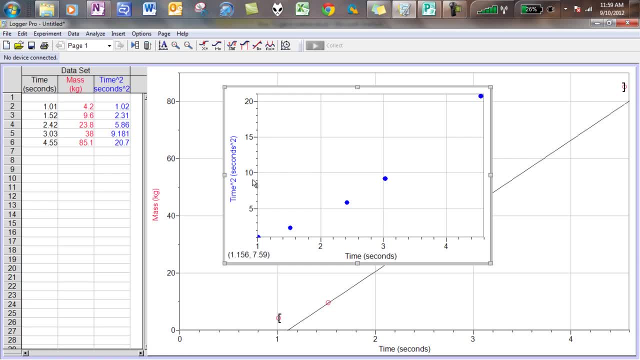 It's not what I want to graph. I want to graph mass versus time squared. So I go on over to where time squared is on my new graph And I want to. it says: click to choose Y column. So I click And you'll notice that I can now select mass. 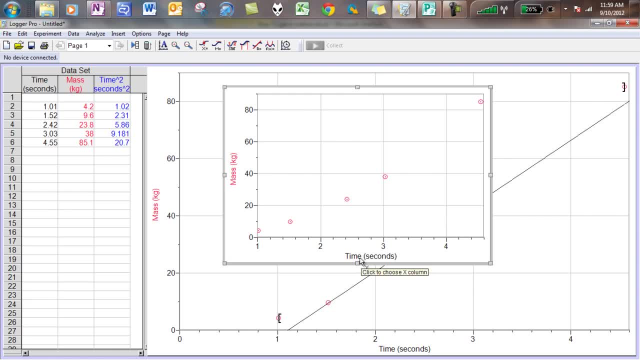 So now I have mass versus time. That's the exact same graph that I had before. So I have to click again And I have to choose time squared, And when I do that, oh, look at that thing, A perfect straight line. 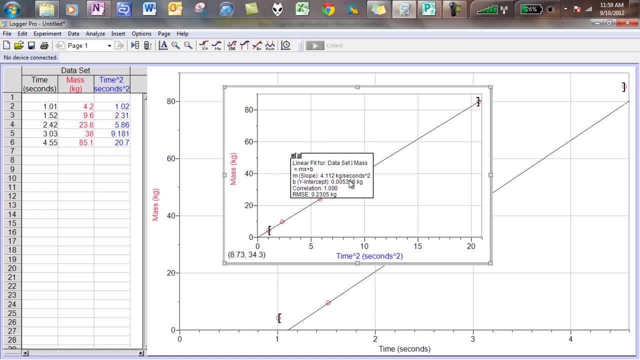 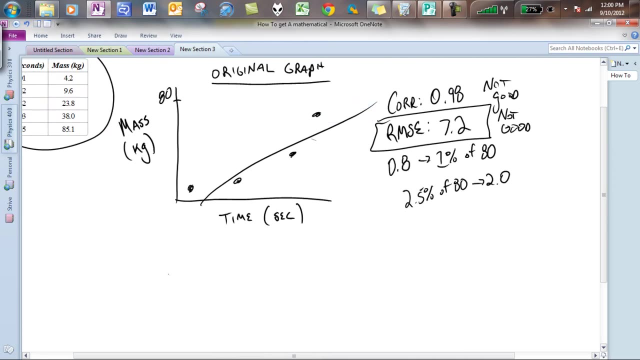 It just looks gorgeous If I hit R equals. oh, it makes me feel so good when you see a correlation of 1.. And so I'm going to actually want to now go back into my document and draw this out. So document changes a little bit, though, because now, if we look at our original graph, 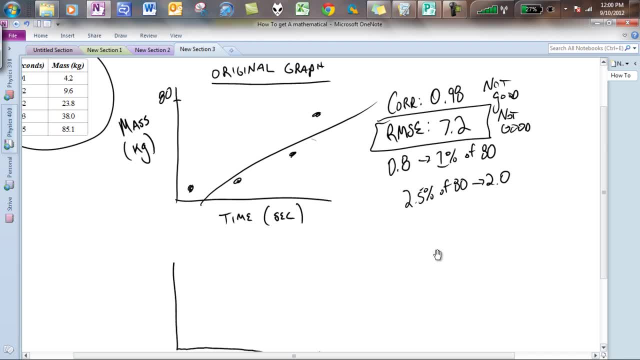 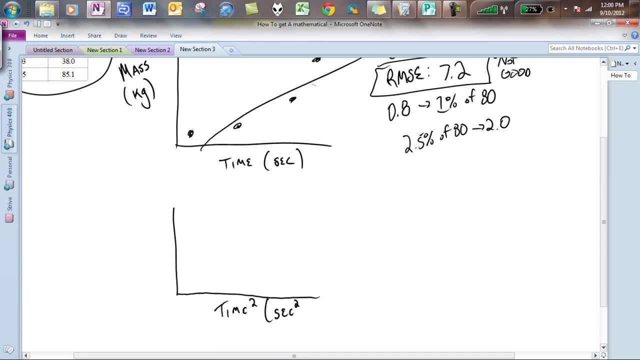 our new graph is going to be labeled a little bit different. This is going to be time squared in seconds squared. So again, we squared both of those. This is mass still in kilograms, And I'm going to draw in those nice, beautiful points that were all nice and straight. 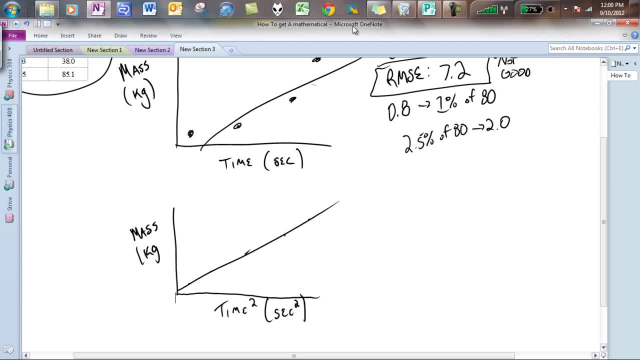 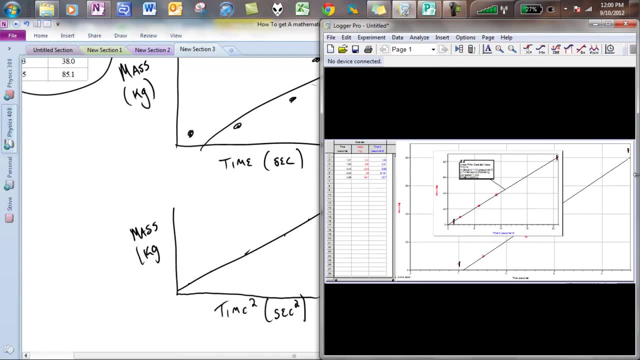 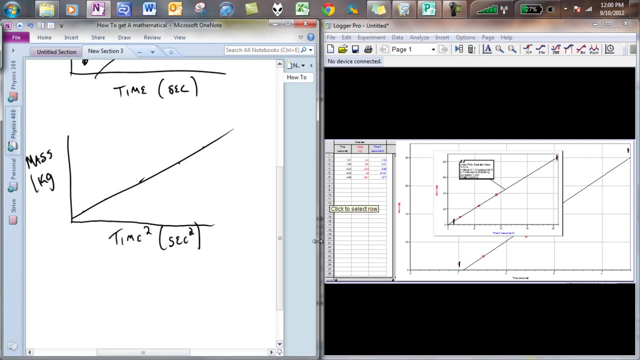 Best fit line there, And then I'm going to write in all of the values that I got from here. So actually, let's make this a little bit easier. Let's put that on over there, Put this on over here. Oh man, it's not going to work unless I can just make this extremely large sheet. 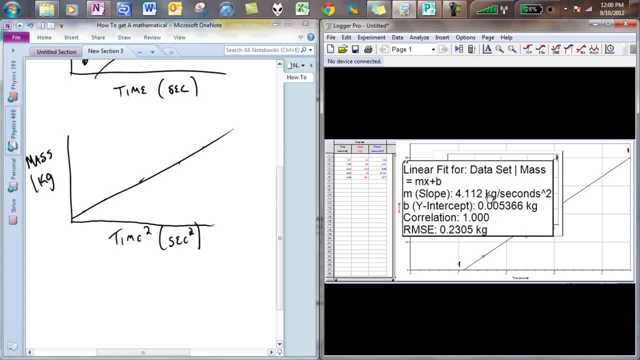 Here we go, All right. So that's all of our stuff from our linear fit. So on over here, Let me just read this, Let me just write those things out. I have m as being 4.112 kilograms per second squared. 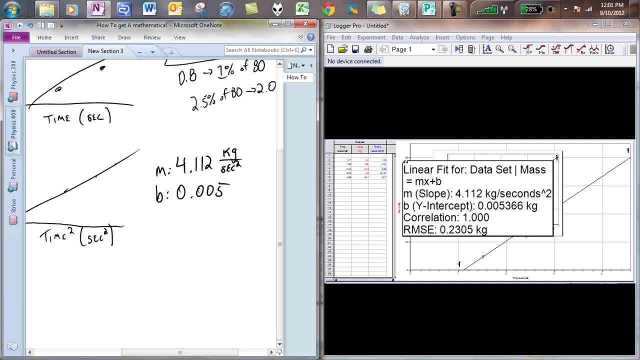 So b is going to be 0.005.. That's in kilograms, And then correlation is a perfect 1.. So we don't even have to do any analysis on that. RMSE will be something that we will have to look at. 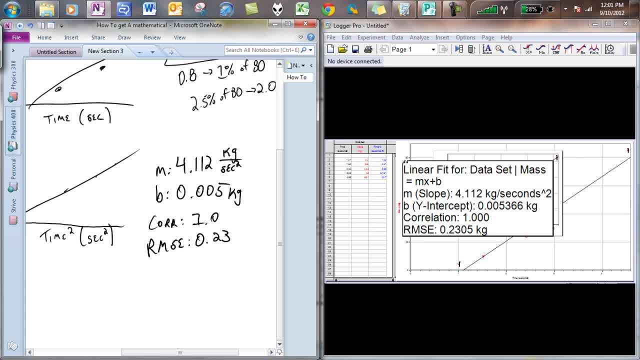 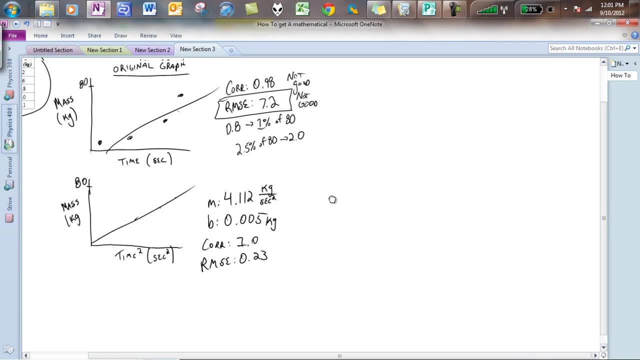 0.23.. Let's double check just to make sure. And my highest value in here is still 80 because of course the y-axis did not change in this case, So we can minimize that. Let's blow this thing up. 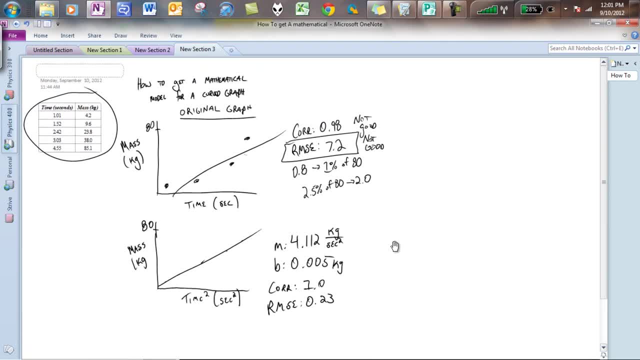 And so if I look at these two graphs side by side, you'll notice that my RMSE has dropped substantially. That's a good thing. Of course, I still want to compare it to 2.5%, So 2.5% of 80.. 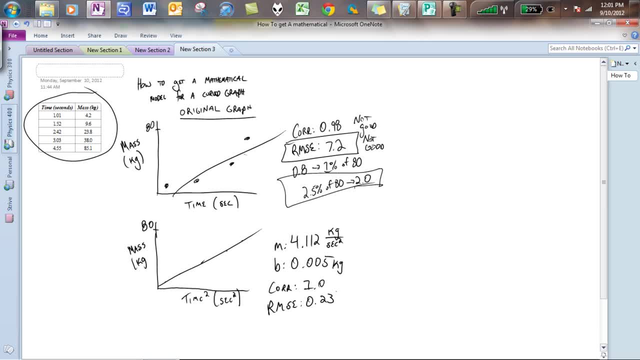 2.5% of 80 is still 2.. So that still falls under. And now you'll notice my RMSE is lower than that. So this is okay. Correlation of 1.. Perfect, We're going to write okay there. 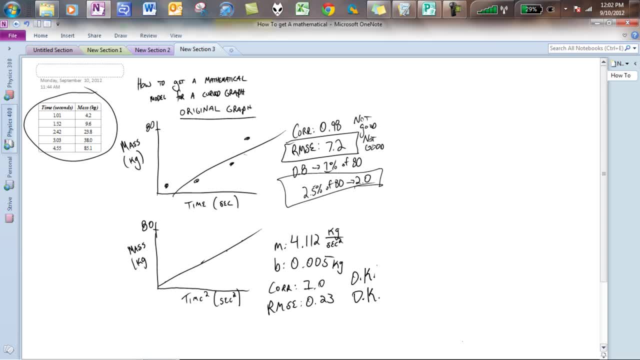 It looks like a straight line And right now you can even look at the y-intercept At time equals 0, does it make sense that I have no mass? Well, I don't necessarily know the experiment, But if I could come up with an experiment that that does make sense, yeah, it probably would. 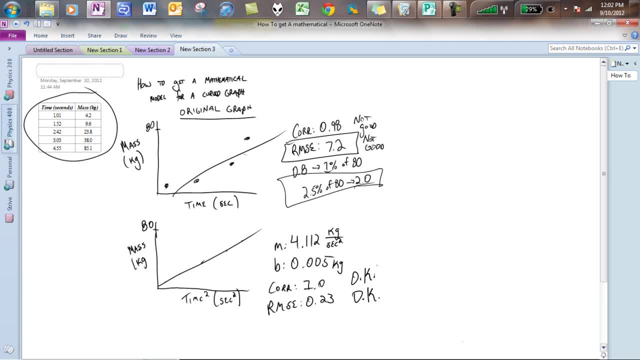 No mass at the beginning and then the mass just continuously increased as time went on. So that would make sense. So now I have to follow my mathematical model And of course I picked the mathematical model from the straight line graph And we know the second one is a better graph. 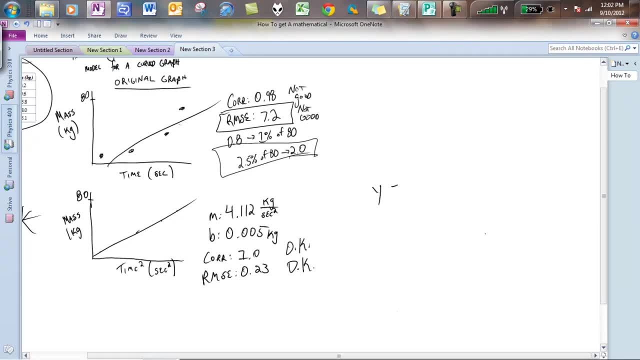 So we're going to use that one And of course I write out what I know is: y equals mx plus b. But this is where people struggle. Remember: y and x are variables, m and b are numbers. Numbers get units. 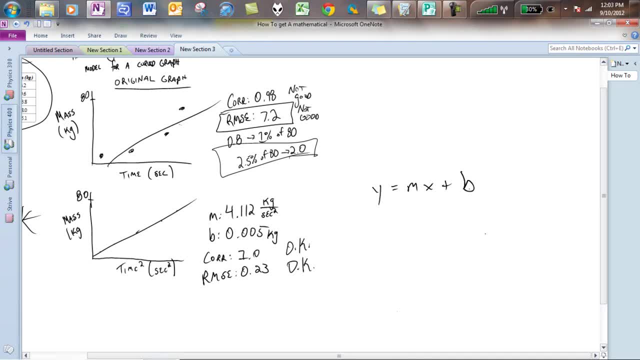 Variables do not. Should I leave y and x in there? No, I should have actual scientific terms. So y is referring to the variable on the y-axis. So I'm going to want to look here and just look at mass. It is not mass in kilograms. 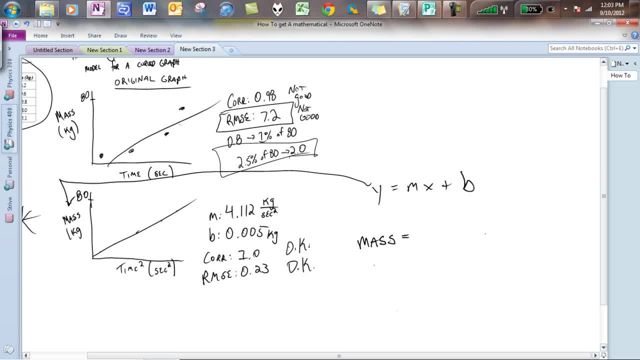 It is just the variable. Do not put what this is measured in, It's just a variable. m is going to be the 4.3., The 4.112,, of course, have units attached with it, So that will be nice. 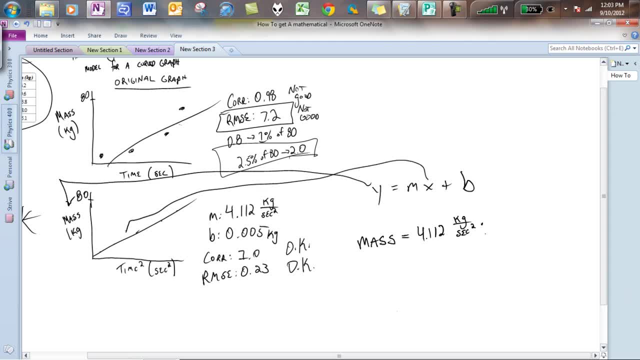 Times. well, it's x, So whatever appears on the x-axis, I look there and I see times squared. So times squared goes there. And then the y-intercept. Well, I'm going to put it in here, But as we go through experiments, I want you to realize that maybe we would want to throw this out. 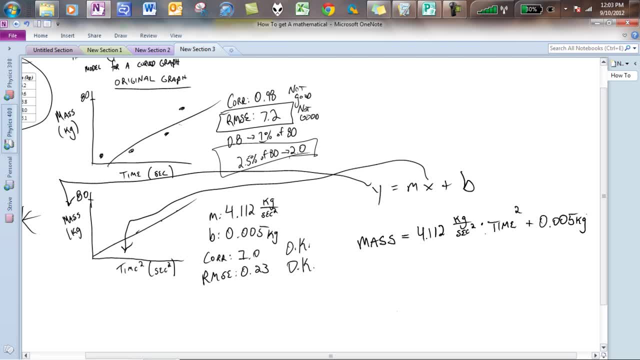 Because it doesn't make any sense, But because I don't know this experiment, I'm going to keep it in there. So we're going to say it's 0.005.. Notice the units that are with it. So, in terms of color, let's just make this really nice and neat. 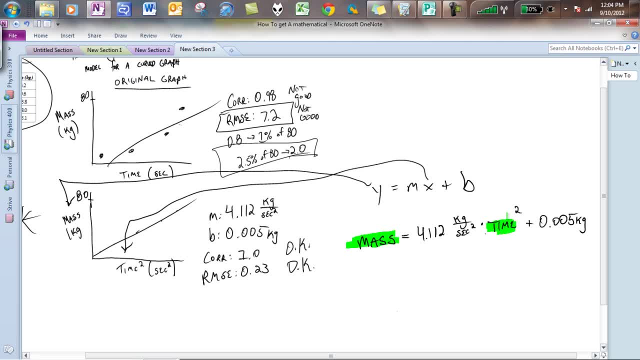 Variables are green, So variables are referring to the y and the x Units. of course will be something a little bit different. Let's call that here, So I'm sorry. numbers get units, Numbers get units, So anything like that. those are two numbers. 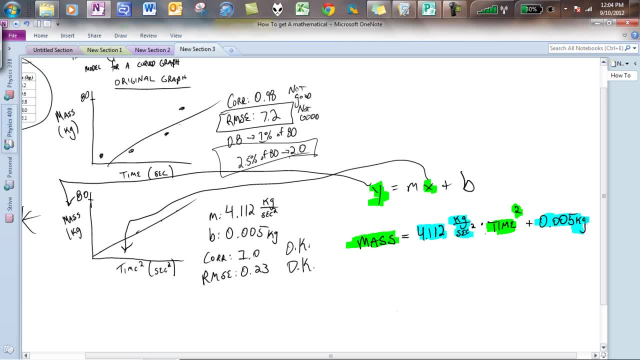 They were referring to units. They will always be the m and the b. Do not leave naked numbers. Make sure our variables are only variables, without any units. So this is our proper mathematical model. This is how you do it And again, I'm going to expect you to do it for the test. 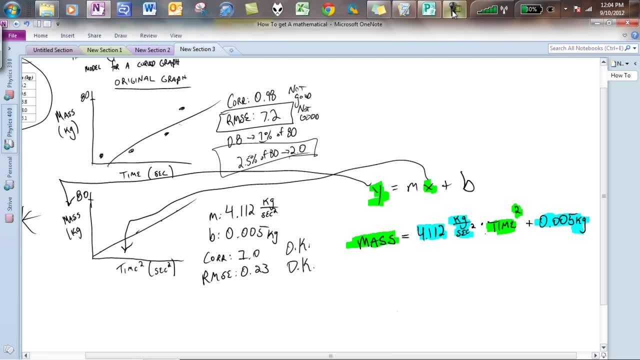 If you have any questions, make sure you ask. Have a great day. Bye-bye.